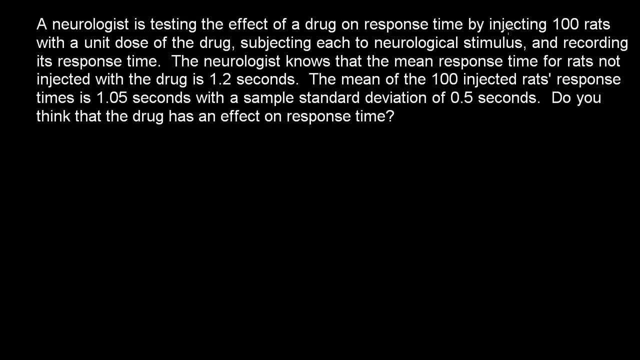 A neurologist is testing the effect of a drug on response time by injecting 100 rats with a unit dose of the drug, subjecting each to neurological stimulus and recording its response time. The neurologist knows that the mean response time for rats not injected with the drug is 1.2 seconds. 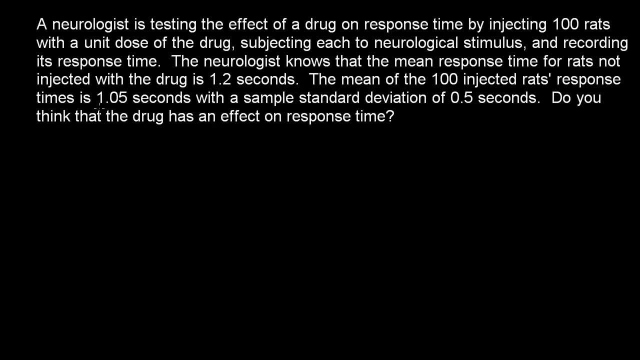 The mean of the 100 injected rats' response times is 1.05 seconds, with a sample standard deviation of 0.5 seconds. Do you think that the drug has an effect on response time? So to do this, we're going to set up two hypotheses. 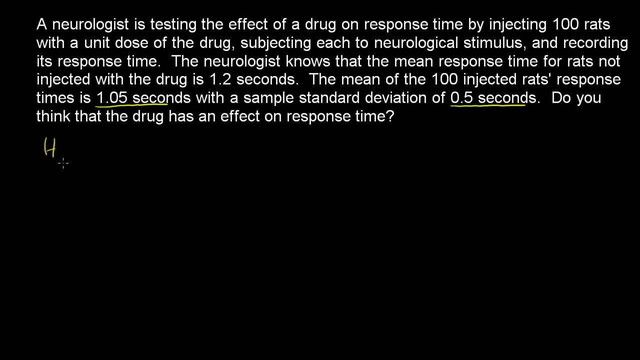 We're going to say the first hypothesis is, we're going to call it the null hypothesis, And that is that the drug has no effect on response time And your null hypothesis is always going to be. you can view it as the status quo. 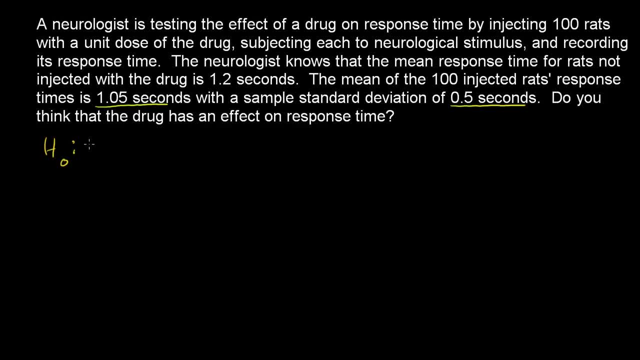 You assume that whatever you're researching has no effect. So drug has no effect. Or another way to think about it is that the mean of the rats taking the drug should be the mean with the drug with the mean. So the drug is still going to be 1.2 seconds, even with the drug. 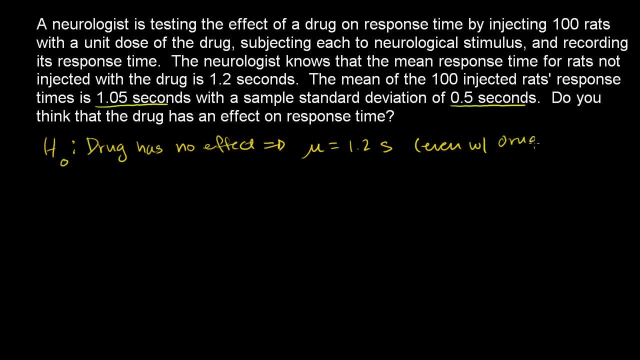 So that's essentially saying it has no effect, because we know that if you don't give the drug, the mean response time is 1.2 seconds. Now what you want is an alternative hypothesis. The hypothesis is no. I think the drug actually does do something. 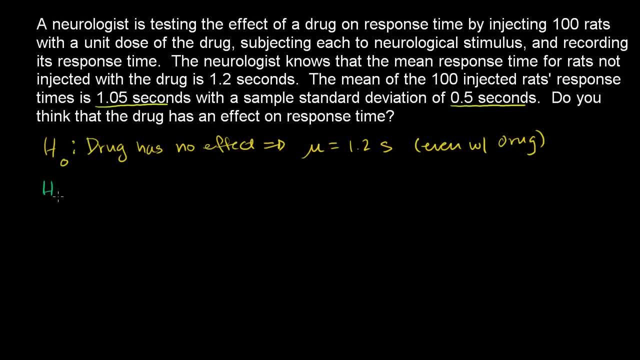 So the alternative hypothesis right over here is that the drug has no effect. It's just that the drug has an effect. Or another way to think about it is that the mean does not equal 1.2 seconds when the drug is given. 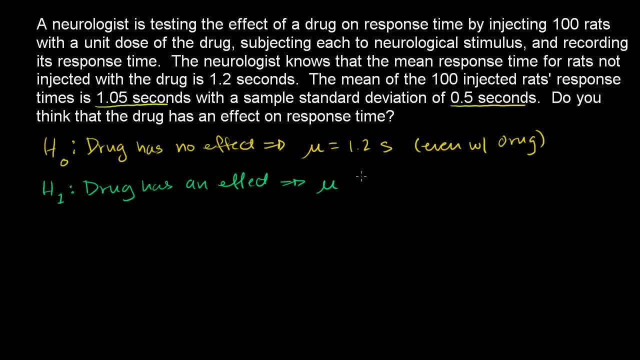 So how do we think about this, How do we know whether we should accept the alternative hypothesis or whether we should just default to the null hypothesis, is because the data isn't convincing, And the way we're going to do it in this video. 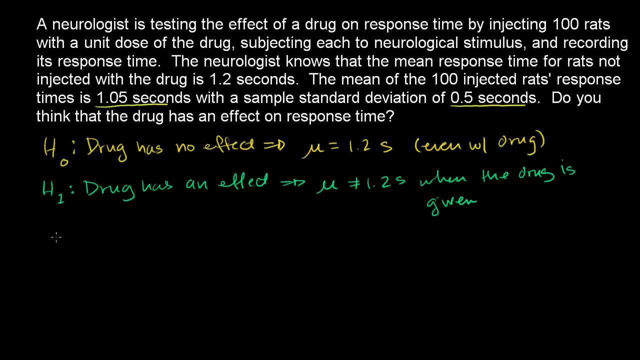 and this is really the way it's done in pretty much all of science, is you say, OK, let's assume that the null hypothesis is true? If the null hypothesis was true, what is the probability that we would have gotten these results with the sample? 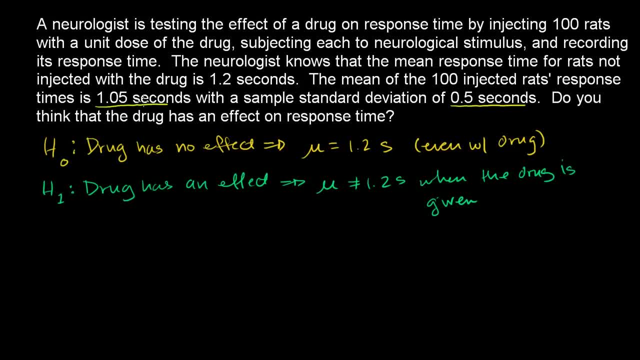 And if that probability is really really small, then the null hypothesis probably isn't true. We could probably reject the null hypothesis and we'll say: well, we kind of believe in the alternative hypothesis. So let's think about that. Let's assume that the null hypothesis is true. 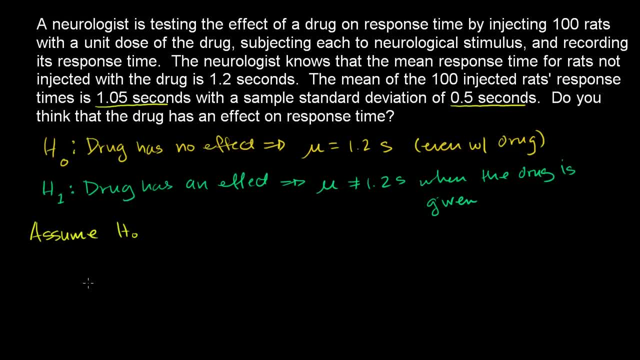 And so, if we assume the null hypothesis is true, let's try to figure out the probability that we would have actually gotten this result, that we would have actually gotten a sample mean of 1.05 seconds with a standard deviation of 0.5 seconds. 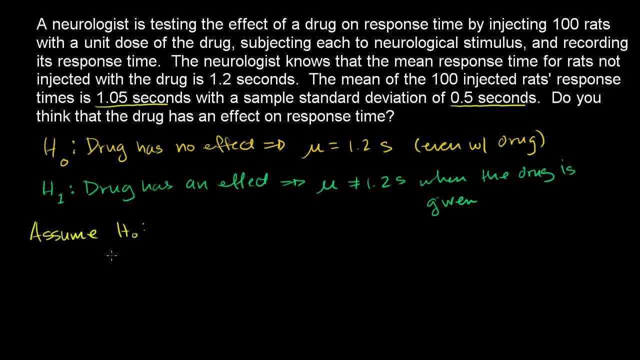 So I want to see if we assume the null hypothesis is true. I want to figure out. I want to figure out The probability and actually what we're going to do is not just figure out the probability of this, the probability of getting something like this. 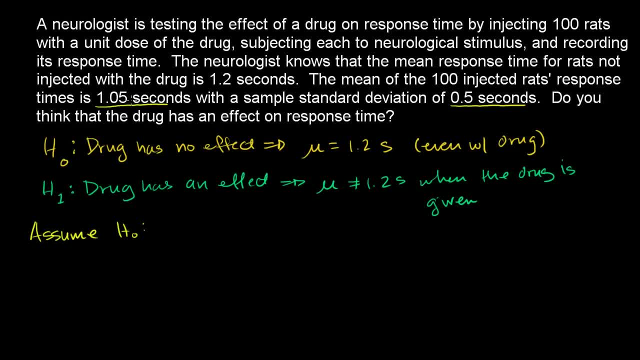 or even more extreme than this. So how likely of an event is that? And to think about that, let's just think about the sampling distribution, if we assume the null hypothesis. So the sampling distribution is like this: It'll be a normal distribution. 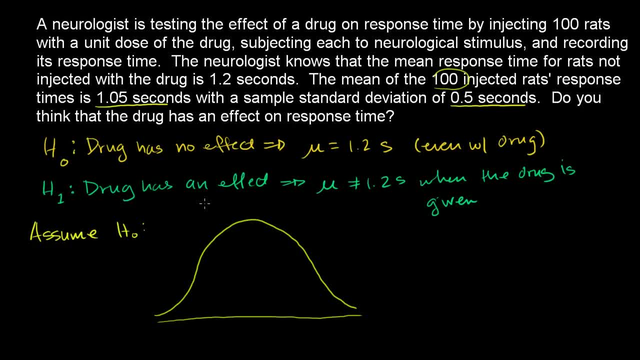 We have a good number of samples. We have 100 samples here. So this is the sampling distribution. We have a mean And now, if we assume the null hypothesis that the drug has no effect, the mean of our sampling distribution will be the same thing. 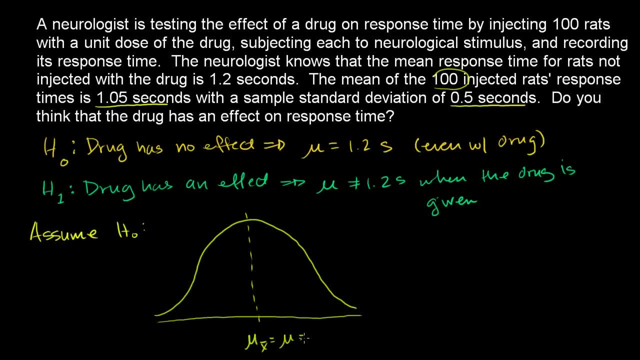 as the mean of the population distribution, which would be equal to 1.2 seconds. Now, what is the standard deviation of our sampling distribution? The standard deviation of our sampling distribution should be equal to the standard deviation of the population distribution divided by the square root of our sample size. 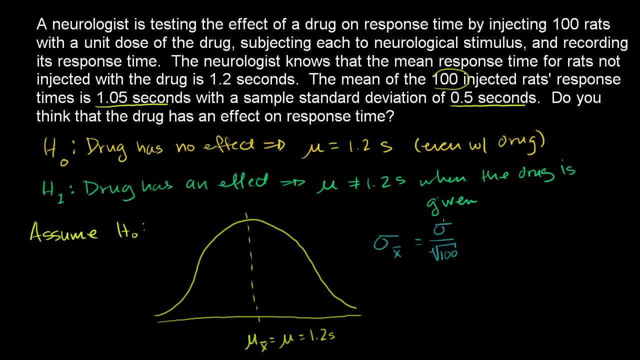 so divided by the square root of 100.. We do not know what the standard deviation of the entire population is, So what we're going to do is estimate it with our sample standard deviation, And that's a reasonable thing to do, especially because we have a nice sample size, a sample 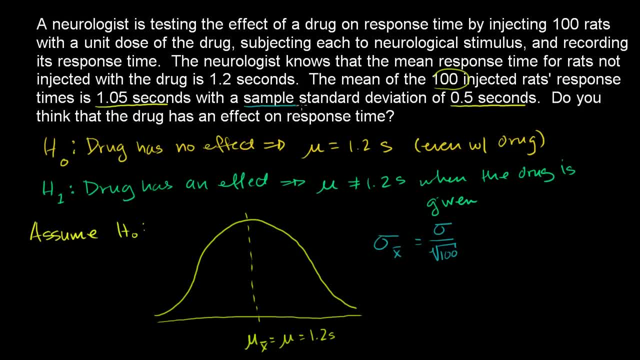 size greater than 100.. So this is going to be a pretty good approximator for this over here. So we could say that this is going to be approximately equal to our sample standard deviation divided by the square root of 100, which is going to be equal to our sample standard deviation is. 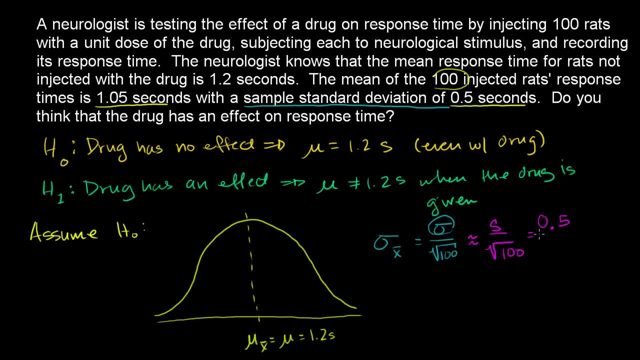 0.5 seconds And we want to divide that by square root of 100 is 10.. So 0.5 divided by 10 is 0.05.. So the standard deviation of our sampling distribution is going to be. I will put a little hat over it to show. 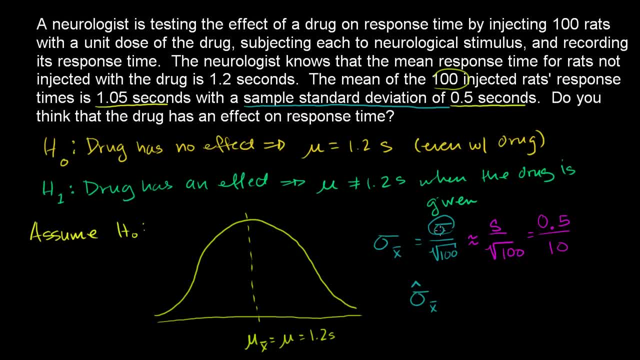 that we approximated the population standard deviation with the sample standard deviation. So it is going to be equal to 0.5 divided by 10, so 0.05.. And so what is the probability? So let's think about it this way: 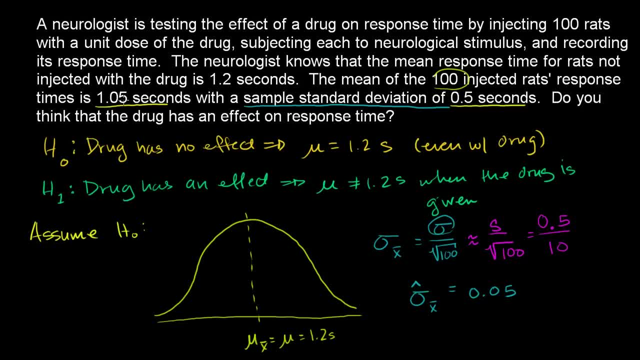 What is the probability of getting 1.05 seconds? Or another way to think about it is: how many standard deviations away from this mean is 1.05 seconds And what is the probability? What is the probability of getting a result at least? 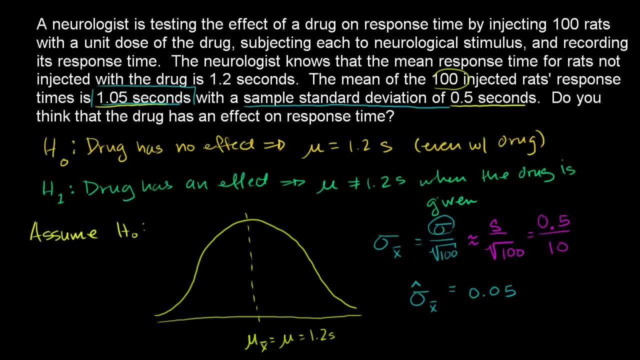 that many standard deviations away from the mean. So let's figure out how many standard deviations away from the mean that is, And essentially we're just figuring out a z-score for this result right over there. So let me pick a nice color. 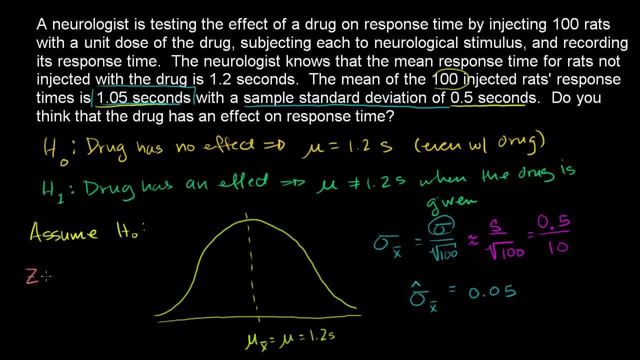 I haven't used orange yet. So our z-score, you could even view it as a z-statistic- It's being derived from these other sample statistics. So our z-statistic, how far are we away from the mean? Well, the mean is 1.2, and we are at 1.05,. 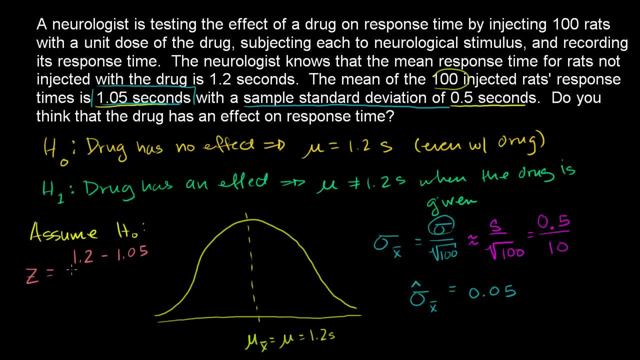 so I'll put that less, just so that it'll be a positive distance. So that's how far away we are, And if we want it in terms of standard deviations, we want to divide it by our best estimate of the sampling distribution's sample standard deviation. 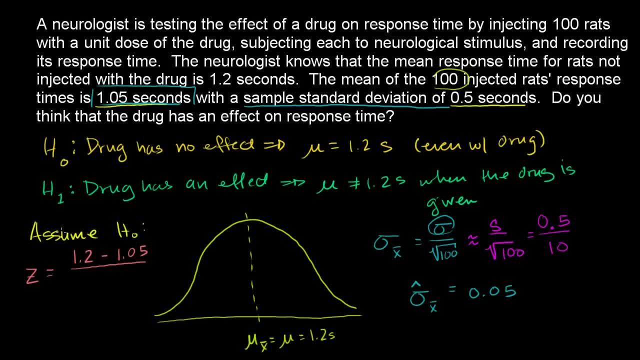 which is this: 0.05.. So this is 0.05.. And what is this going to be equal to? z this result right here: 1.05 seconds. 1.2 divided by 1.2 minus 1.05 is 0.15.. 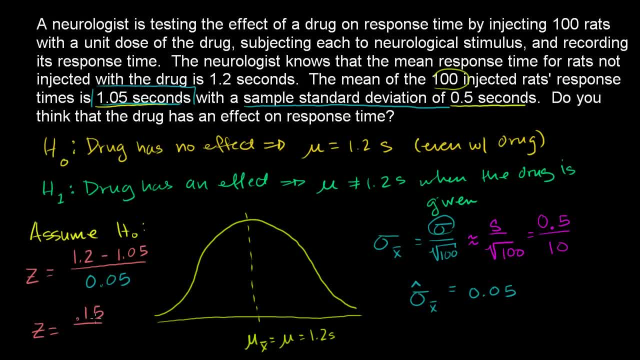 So this is 0.15 in the numerator divided by 0.05 in the denominator, And so this is going to be 3.. So this result right here is 3 standard deviations. So let me draw this. This is the mean. 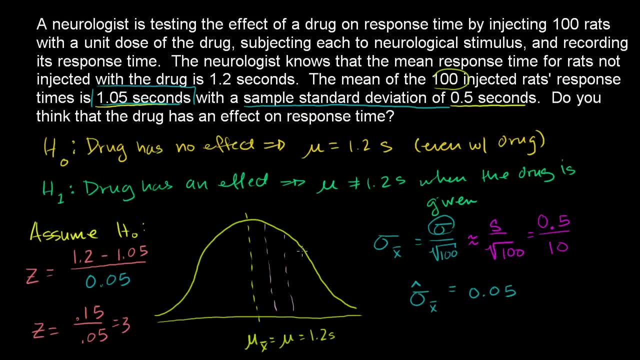 If I did one standard deviation, two standard deviations, three standard deviations, that's in the positive direction. Actually, let me draw it a little bit different than that. This wasn't a nicely drawn bell curve, but I'll do one standard deviation. 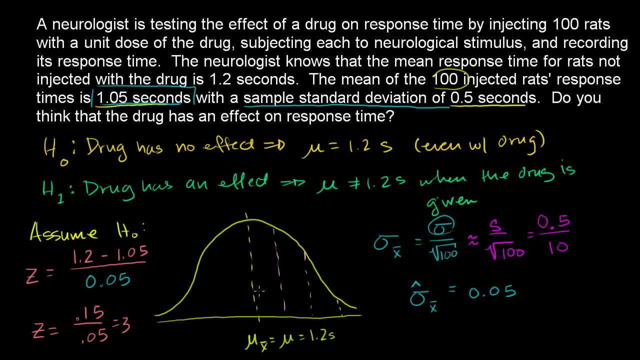 two standard deviations and then three standard deviations in the positive direction. And then we have one standard deviation, two standard deviations and three standard deviations in the negative direction. So this result right here, 1.05 seconds that we got for our 100 rat sample is right over here. 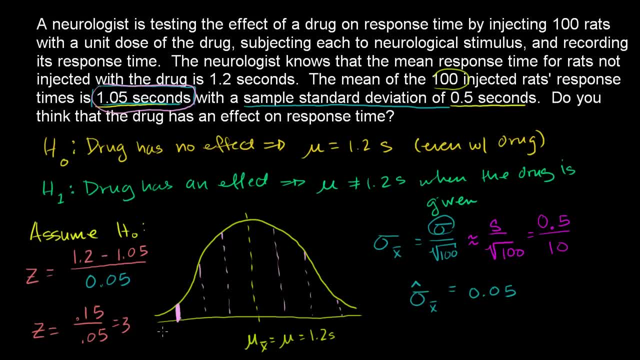 Three standard deviations below the mean. Now, what is the probability of getting a result this extreme by chance? And when I talk about this extreme, it could be either a result less than this or a result that extreme in the positive direction, more than three standard deviations. 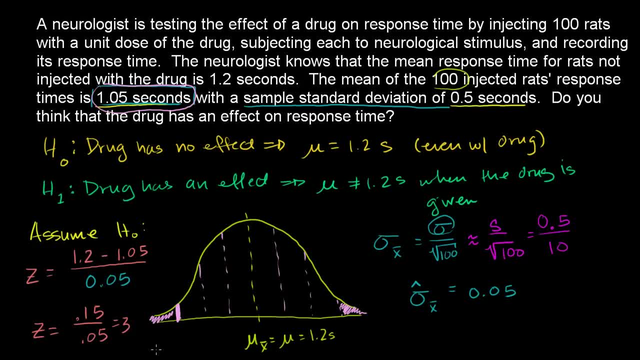 So this is essentially, if we think about the probability of getting a result more extreme than this result right over here. we're thinking about this area under the bell curve, both in the negative direction or in the positive direction. What is the probability of that? 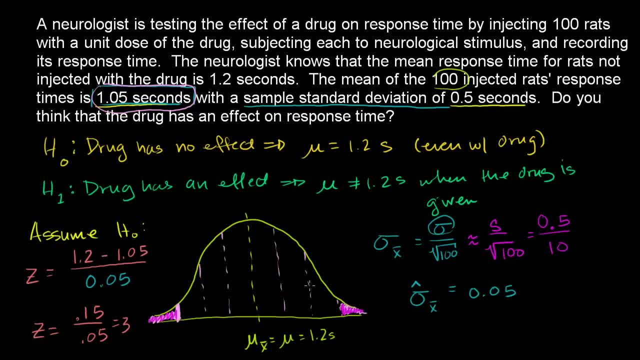 Well, we know from the empirical rule that 99.7% of the probability is within three standard deviations. So this thing right here, you could look it up on a z-table as well. but three standard deviations is a nice, clean number that doesn't hurt to remember. 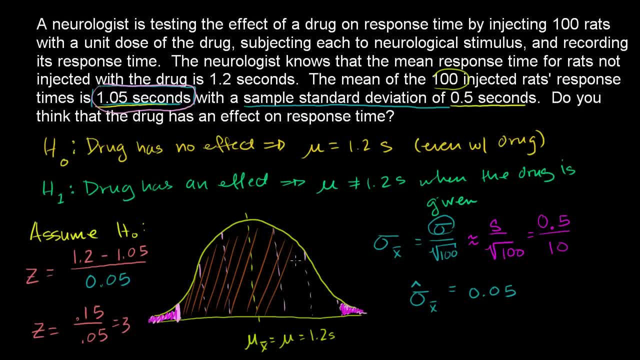 So we know that this area right here- I'm doing in this reddish orange, that area right over there, is 99.7%. So what is left for these two magenta or pink areas? Well, if these are 99.7%, then both of these combined. 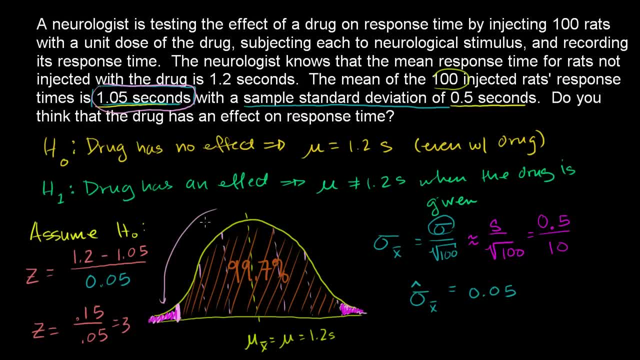 are going to be 0.3%, So both of these combined are 0.3%. I should write it this way: Exactly are 0.3%, 0.3%, 0.3%, Or if we wrote it as a zesimal, it: 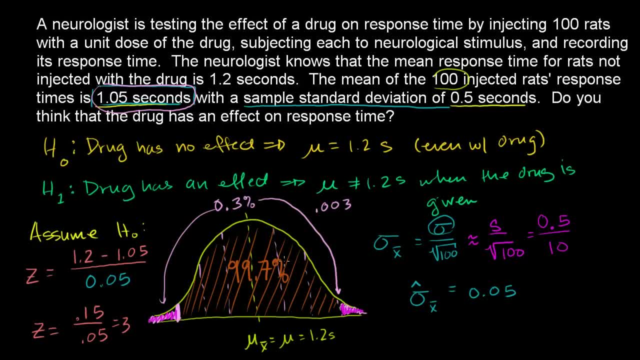 would be 0.003 of the total area under the curve. So, to answer our question, if we assume that the drug has no effect, the probability of getting a sample this extreme, or actually more extreme than this, is only 0.3%, less than 1 in 300.. So if the null hypothesis was true, 0.3% of the total area under the curve- 0.3%- less than 1 in 300.. So if the null hypothesis was true, 0.3% of the total area under the curve- 0.3%- less than 1 in 300.. 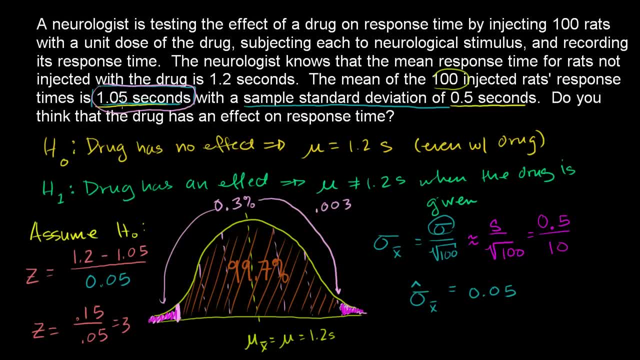 there's only a 1 in 300 chance that we would have gotten a result this extreme or more. So at least from my point of view, this result seems to favor the alternative hypothesis. I'm going to reject the null hypothesis. I don't know 100% sure, but if the null hypothesis was true, 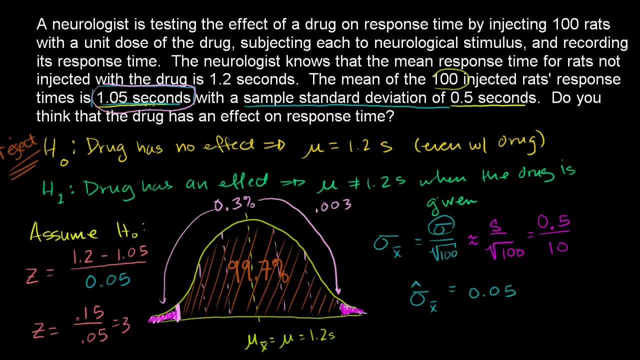 there's only a 1 in 300 chance of getting this, So I'm going to go with this, The alternative hypothesis, And just to give you a little bit of some of the name or the labels you might see in some statistics or in some research papers, this value. 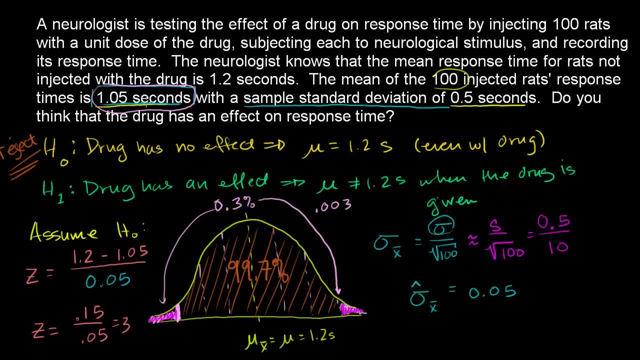 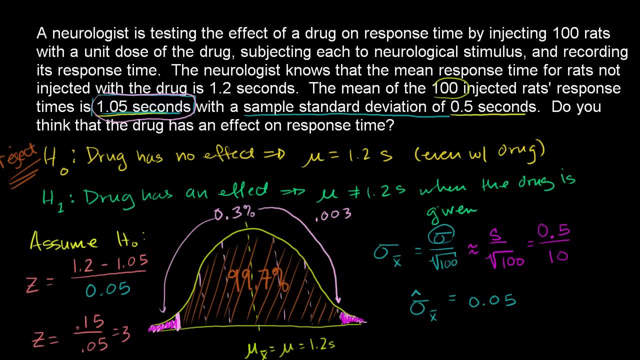 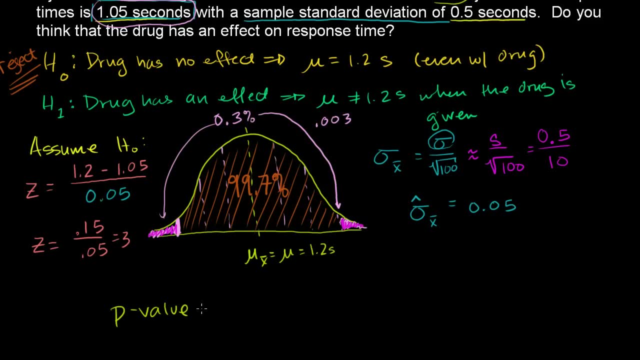 the probability of getting a result more extreme than this, given the null hypothesis, is called a p-value. So the p-value here, and it really just stands for probability value, is called a p-value. So the p-value here, and it really just stands for probability value. 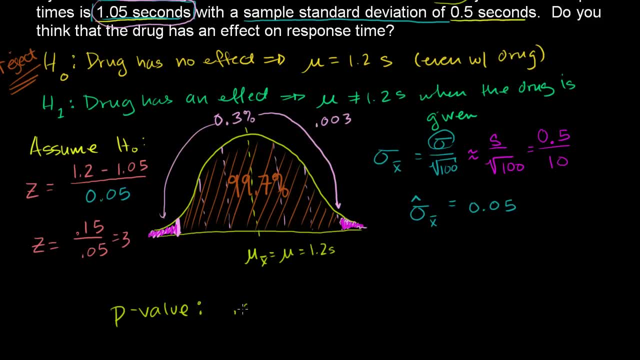 the p-value right over here is 0.003.. So there's a very, very small probability that we could have gotten this result if the null hypothesis was true. So we will reject it And in general, most people have some type of a threshold here. 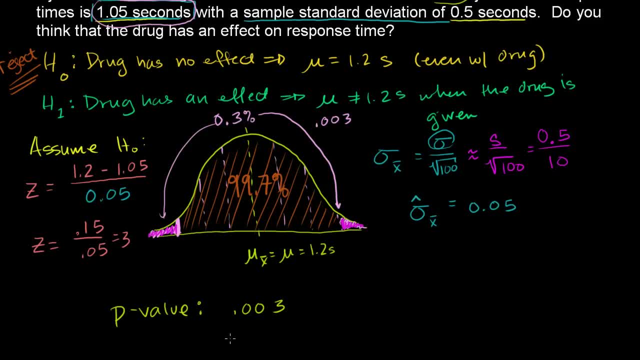 If you have a p-value less than 5%, which means less than 1 in 20 shot, they'll say: you know what? I'm going to reject the null hypothesis. There's less than a 1 in 20 chance of getting that result.